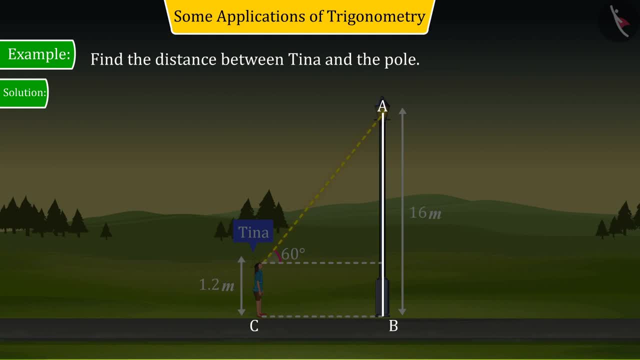 And let's also assume that the distance between Tina and the pole is BC, where the measurement of BC is represented by X meters. Since we have to find the horizontal distance between Tina and the pole, draw a horizontal line relative to Tinas point of view D, which is perpendicular to AB. 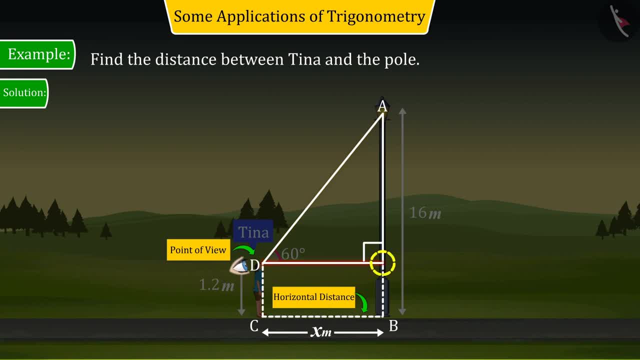 And the point at which it cuts AB. let's represent it by point E, from which we get a new triangle ADE where side DE is parallel and equal to side AC and equal to side AC side CB. In triangle ADE, the elevation angle formed by line of sight and horizontal line. 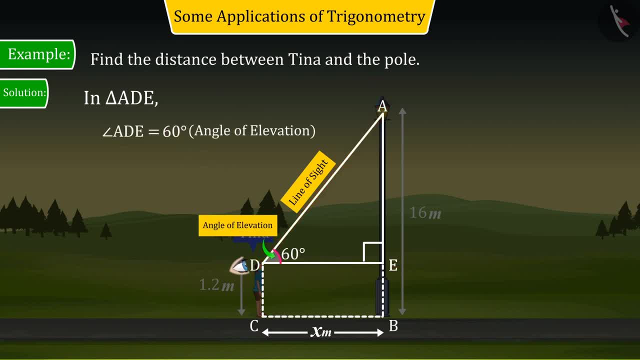 will be ADE and it is of 60 degrees. So with the help of triangle ADE, can you find the value of horizontal distance DE? Let's see. With the help of the information obtained using the trigonometric ratio in triangle ADE, you can tell that the trigonometric ratio 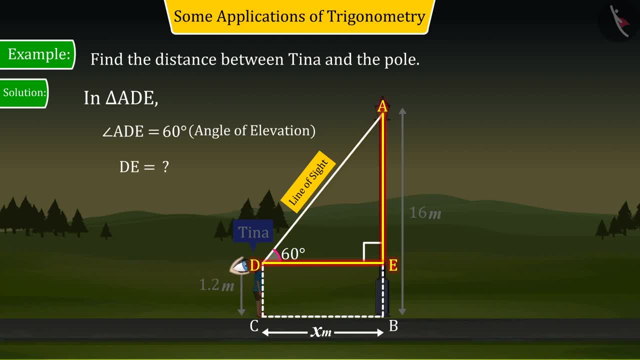 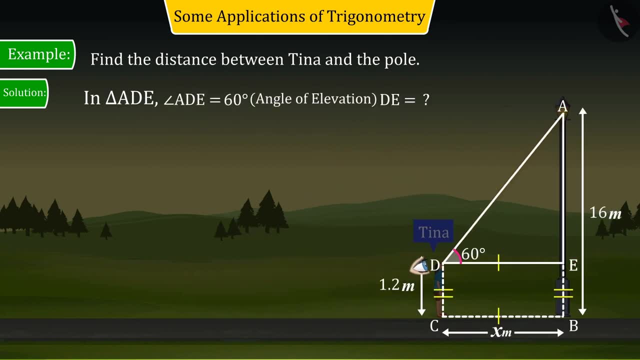 made from the side opposite to and adjacent to angle D will be tan, because here side AE is known, from which the value of tan, 60 degrees, is obtained as AE by DE, Where the measurement of sides AE and DE is 14.5,. 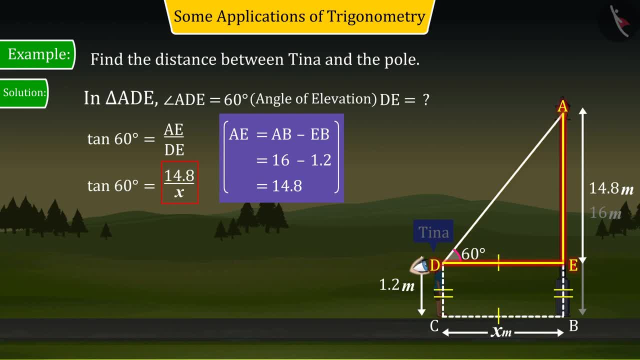 point 8 and x meters respectively, Since CD is parallel and equal to BE and BC is parallel and equal to ED, And we know from the trigonometric ratio table of specific angles that the value of tan, 60 degree, is square root 3.. By solving all these values obtained in the above equation, 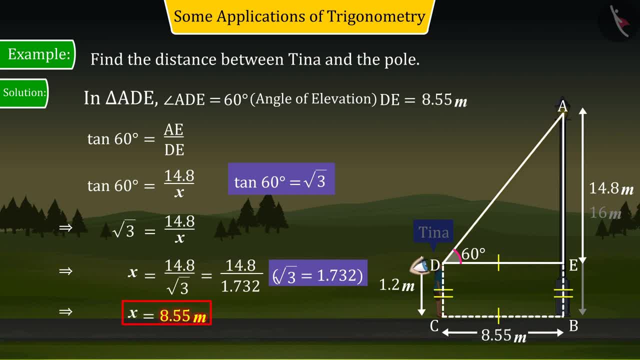 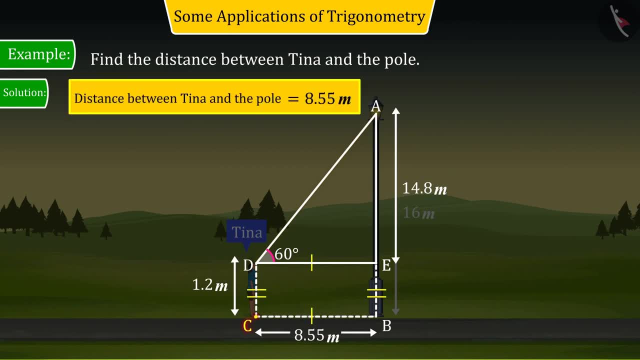 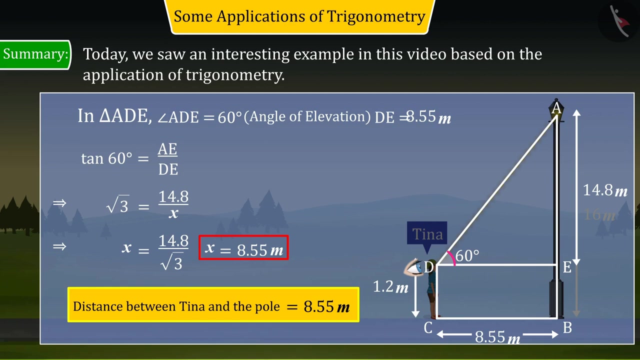 the value of x is obtained as 8.55 meters, With the help of which we can say that the horizontal distance of the pole from the place where TINA is standing is 8.55 meters. Today we saw an interesting example in this video, based on the application of trigonometry.